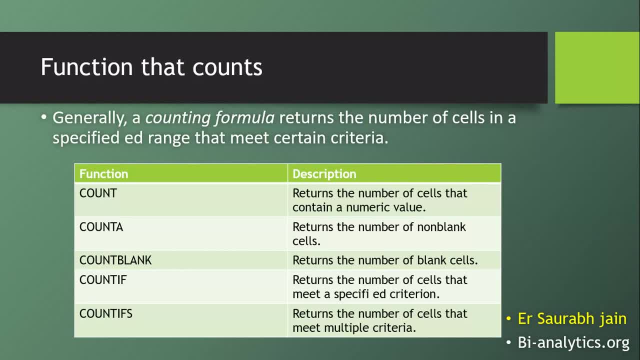 So if the cell has a numerical value, count will count. that cell Count returns the number of non-blank cells. So if there is a cell with numeric or text data, it will count both, so it should not be blank. Then count can be used. Third is: count returns the 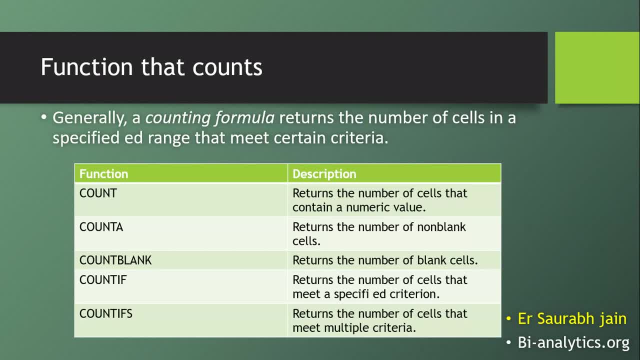 number of blank cells. Then you have a formula called count returns the number of cells that meets a specific criteria. Say count if. if the length is greater than 500 meters, So it will count all the elements which have a length greater than 500 meters. Count ifs. here is a S attached. 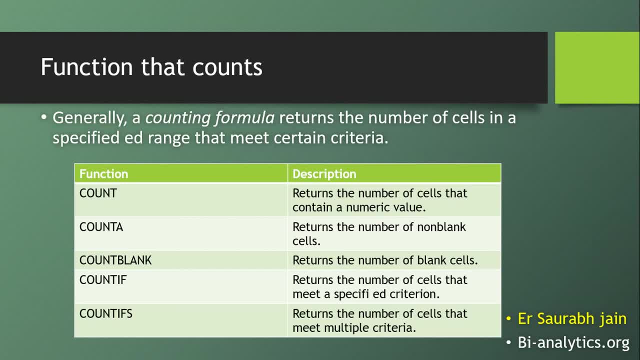 to this formula. This was used in Excel 2007,, I think So. count, ifs is used, returns the number of cells that meets the multiple criteria, So you can have more than one criteria, Say you. say I am looking for a number of elements which have length greater than 500 meters and and whose color 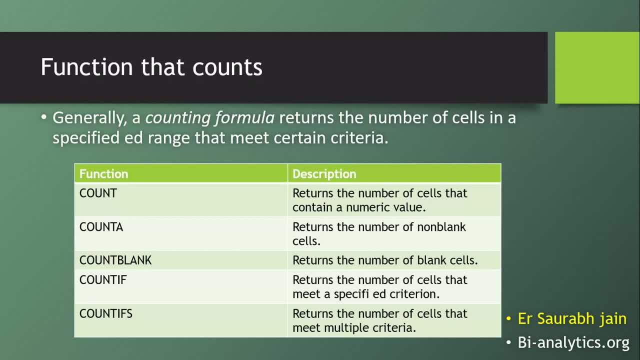 is also red. So you have two criteria. Say, if there is a table with color, length and elements, So you are identifying that color has to be red And secondly, you also want that length has to be greater than 500. So you are counting in that way. So this is the way it's done. So let's start first. 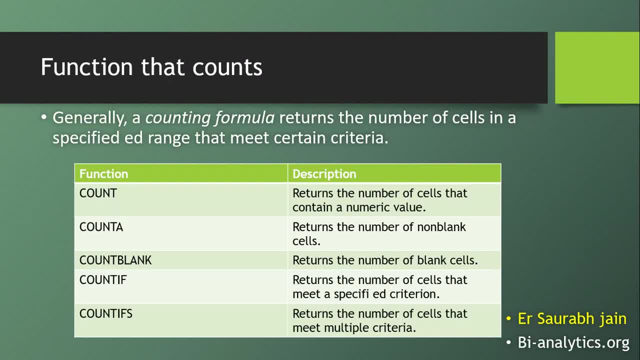 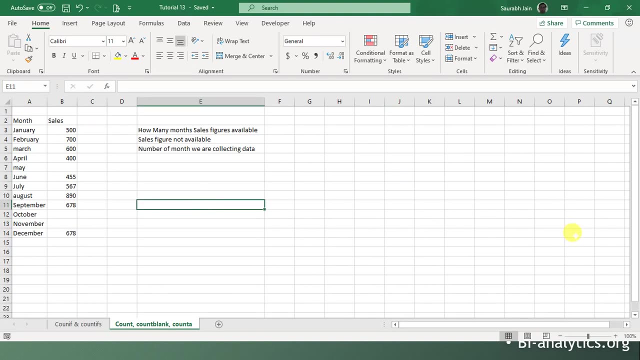 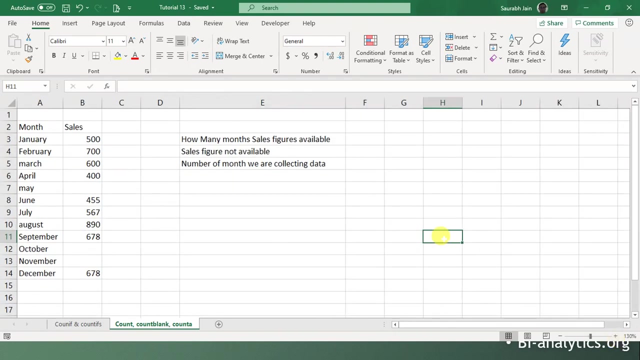 example of count, count a and count blank, And then we'll take another example for count if and to understand how. what is a practical applications? Let's start. So let me take you to the Excel. See, this is a data. Okay, I also have one special request for you all, If you are watching on, 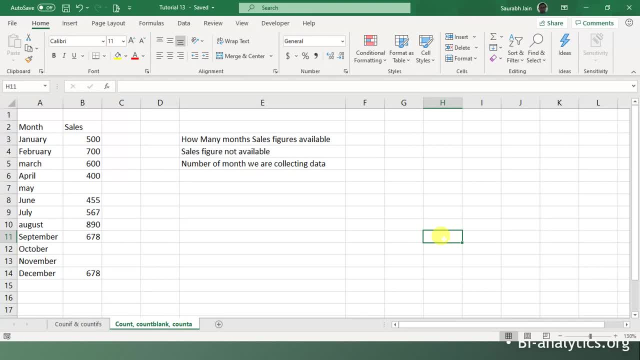 Facebook or YouTube this video. please write your name and location So I will come to understand and what is your current designation, What actually, in which field you are. So that will help me to understand what is my audience and who, who people are looking and. 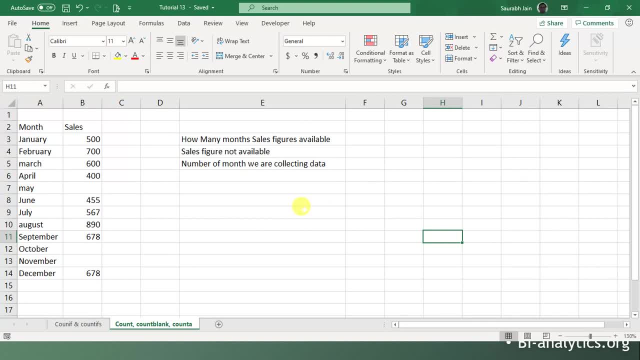 watching my videos and are you liking it or not. This is also important, So let's start. So look, this is a data, This is months and sales. So there's a January, February, 12 months and you have sales. Assume a hypothetical case that I have been given a task to make a report and I am 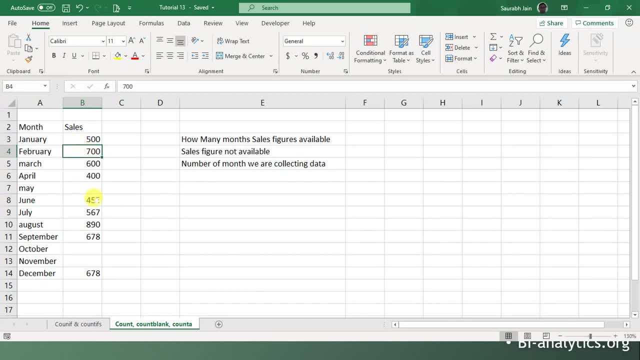 collecting these figures? How many sales have been in the January, February, March, April like this? Fine? So now I need to find out- I have a couple questions- How many months of sales figure available with me? So when it was my task, 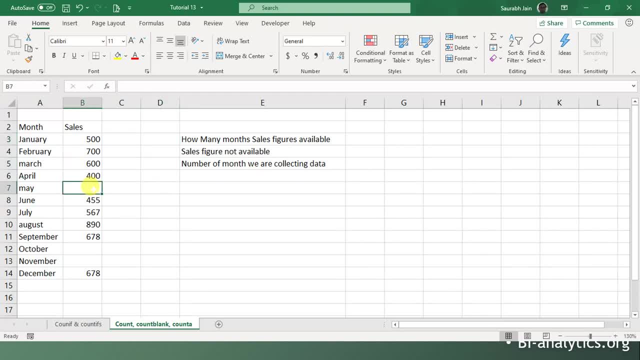 there are. you can see that I still have to find the sales figure of May, which is not available with me. I have to find for October, November. So my question is: how many months of sales figures are available with me? So actually I'm looking for all the data which has numerical value. So 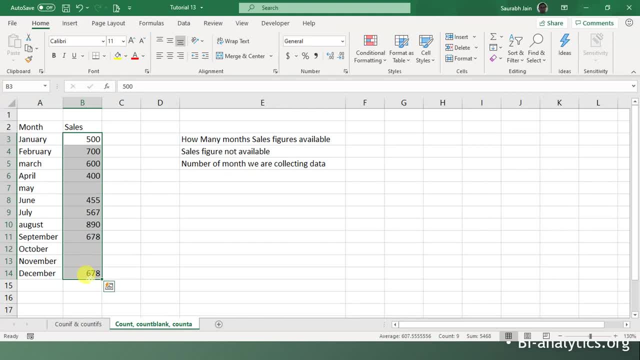 I want to count all the numerical values, events. So let's start. So we'll use simple count formula. I'll write is equals to COUNT and I'll just select this entire range. So I'm counting all numerical values in this particular range. So this is nine. It's telling. 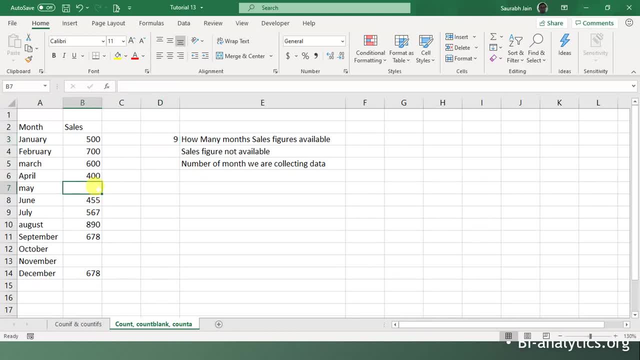 me that nine sales figures have been added. So if I write any over here it will still be show nine, but if I say write 789, it will show 10.. Fine, So hopefully you understand that it will calculate only numerical values. So now next question: sale figures not available, So I need to count all the 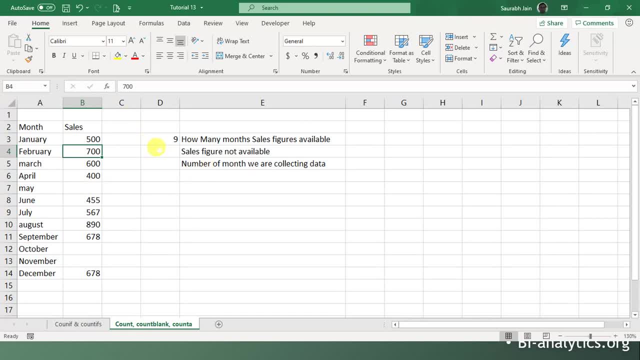 blank cells. So I can see there are three blank cells. So I'll use count. blank is equals to COUNT and BLA and count blank. bracket open And I again select the entire range. bracket close, enter. So I have this. three which are non-blank, Fine. Which are blank, Okay. So this is why we use count blank. 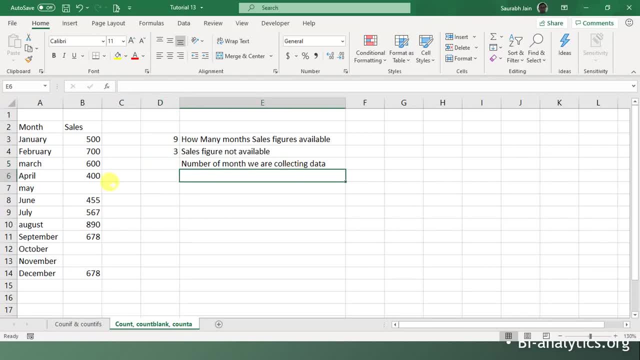 formula. Now, third point: Number of months. we are collecting data, So suppose I want to count how much are these values? It can be text also, It can be numeric also, So I will use count A formula. It will can be used for text also, for numerical also. So let's do it is equals to COUNT. 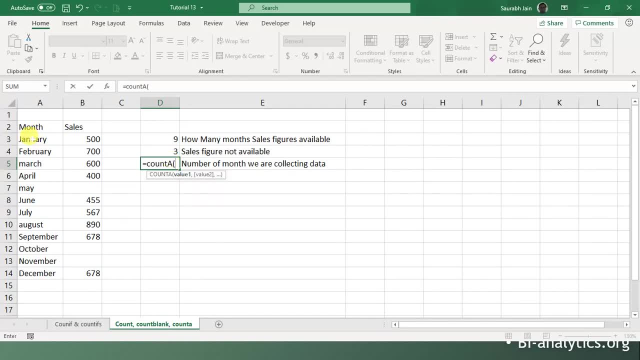 COUNT A bracket open. this time we are taking a different range. Previously it was sales, this time it is months, So let's give me 12.. Fine, So this is the way this has been done. So these were the three formulas. remember: count, count A and count blank. Count will count only. 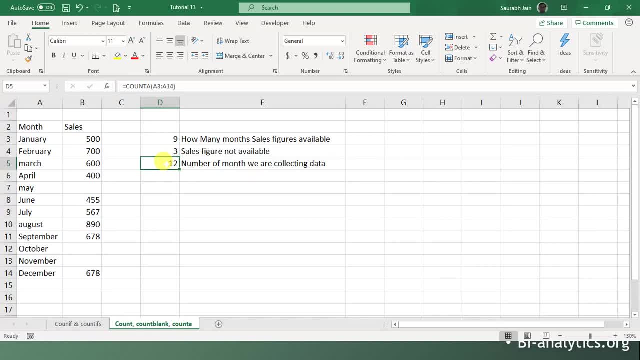 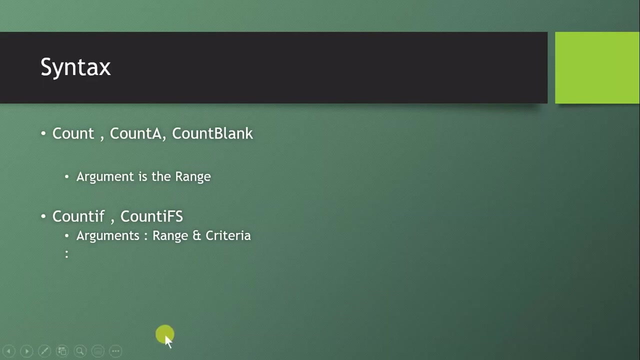 numeric data, fine, and count blank will count number of blanks in the cells. and if you want to count non, which are not blank, then we will use a remember which are not blank will be counted by count a. fine. okay, let's move further. so if you talk about count if and count ifs, you need a range. 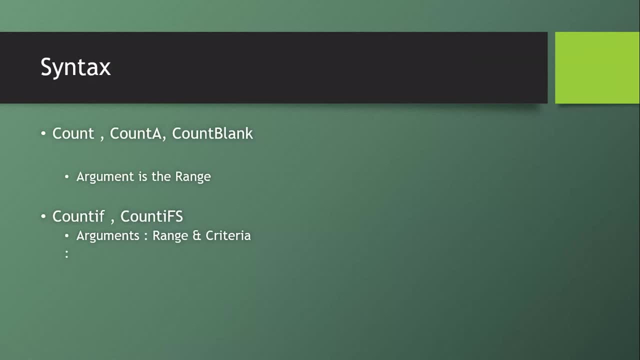 and criteria. range is like: i will be counting in particular range and my criteria will be: color is red, greater than four, less than four, equal to this, something like this. so what i will do is i'll take you an example and we'll have some- around five to seven, ten questions and we'll try to answer. 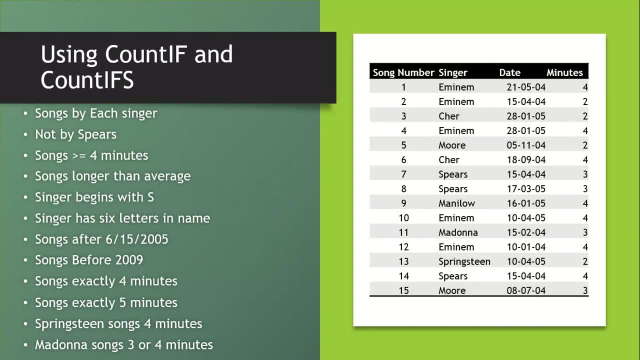 that question from the following database. let's start look. this is my database, which has song number. we have singer like spears, madonna, like this, and they have date on which date they have sung. thirdly, you have minutes four, two, two, two, four, four, four, five. so these are the songs they have sung for particular minute. so we can have questions. 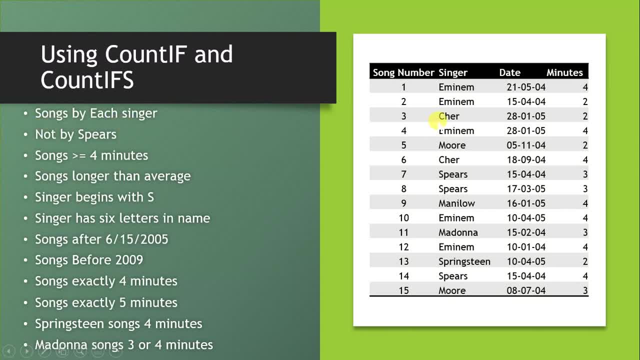 like count number of songs by each singer. so how many songs have been sung by spears? we have to count this, fine, not by spears. so we want to find count all the songs which are not being counted by spears. songs greater than equal to four minutes. song less than: 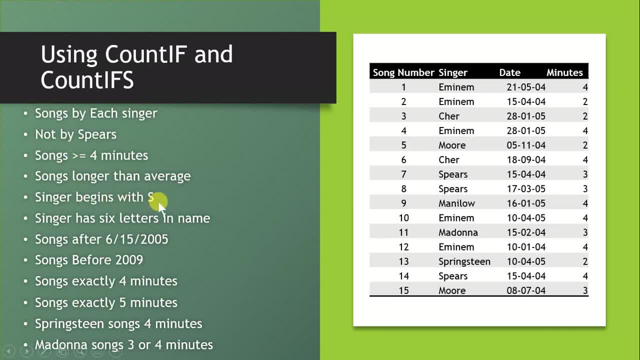 average singer begins with s. we want to identify a singer whose name begin with s singer has six letters in the name, so i want to identify all the singers with six letters in the name. fine songs sung after 6: 15 2015 songs before 2009. songs exactly of four. 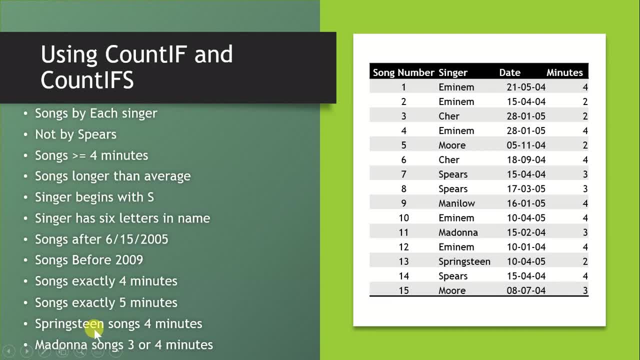 minutes. song exactly of five minutes, springton songs of four minutes, madonna songs for three or four minutes, which means it has been three to four minutes. so these are some questions, so we have to count. so so we have a database ready and we have questions, so let's try to use count if and count ifs formula. 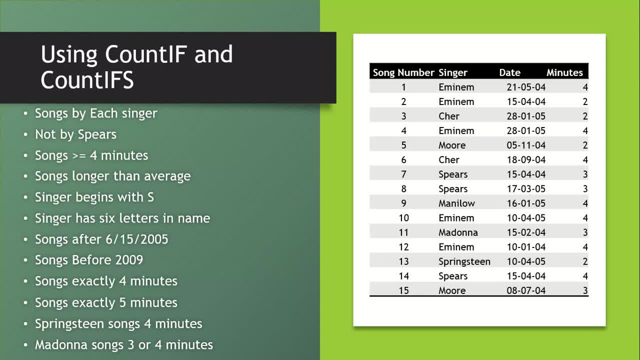 to understand how it will be done. let's go ahead. remember you can download these files from the website. website name is bi-analyticsorg. please download and make sure you also do it, because if if you will just watch it out, you will understand how it is done, but if you will practice with your 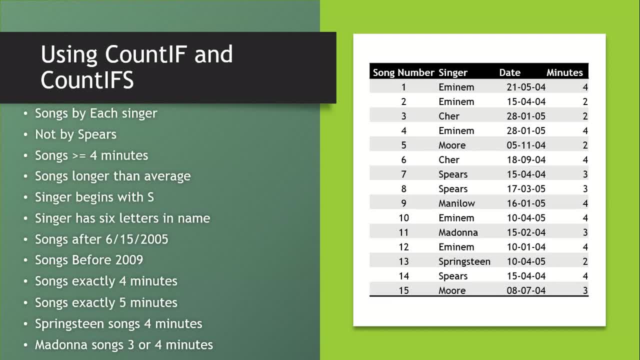 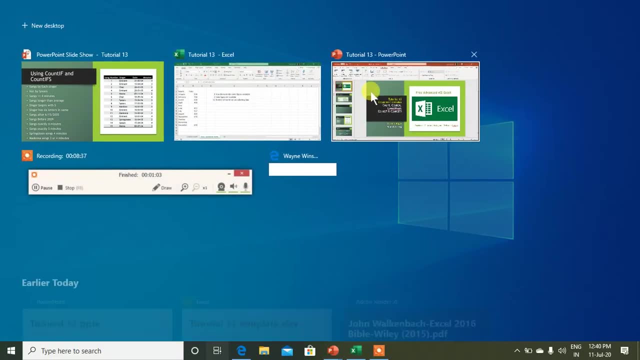 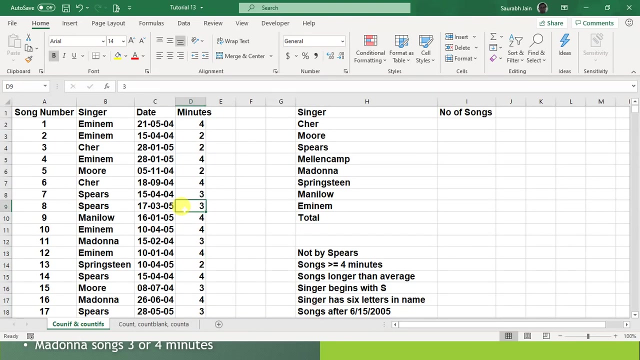 hand, then it will be always be last long with you in your brain. so it is important to do practice. fine, make sure to download the template file. i will share the links of the download files in the link below in the description. let's start. so see, i have this data available with me right now: songs: i have a singer name. i have date. 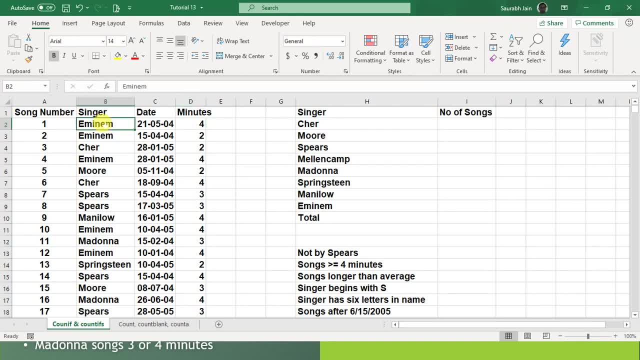 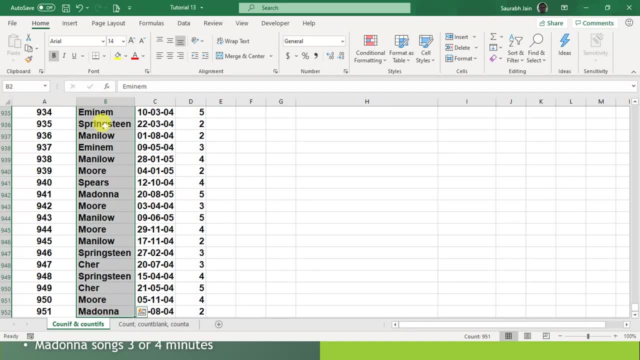 i have minutes, if i. if you want to select a range, remember one thing: ctrl shift down arrow. ctrl shift down arrow. it will take you to help you in selecting the range. so we can see there are total number of 951 songs available. fine, you can see this- 951. okay, i have also seen people watching the mobile- this video: 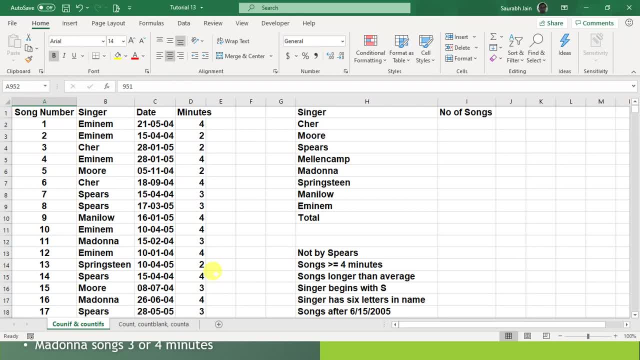 on mobile phones. so if you are watching on mobile phone, please make sure to do full screen. it is important, but then only you will be able to see the numbers. let's start. so look, i have this name of the singers available with me and i want to find number of songs sung by. 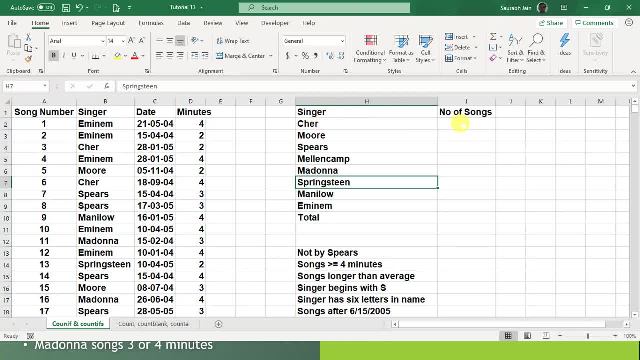 springton madonna chair like this, fine, so i have to apply count if formula i want to count if all the values, if the name is chair, fine, so let's start you- is equals to c, o, u and t count if it is a single criteria. there's no multiple criteria in this. 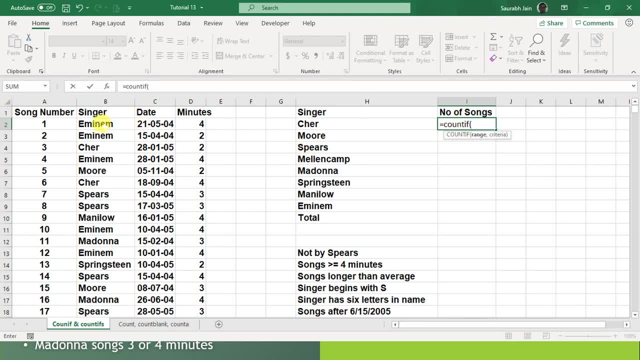 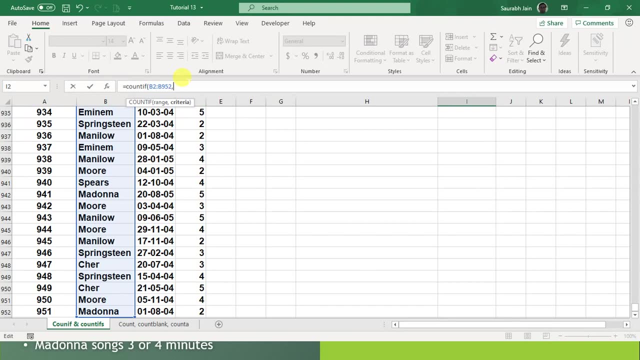 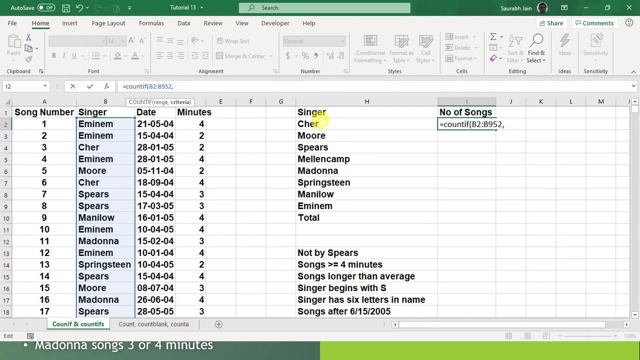 so bracket open, i say i have to count from this cell and i forget to tell you that i have to do ctrl, shift, enter. so this is my cell collected comma. now i have to type the name of the person who's i am looking forward. so what i can do is i can just select this also. 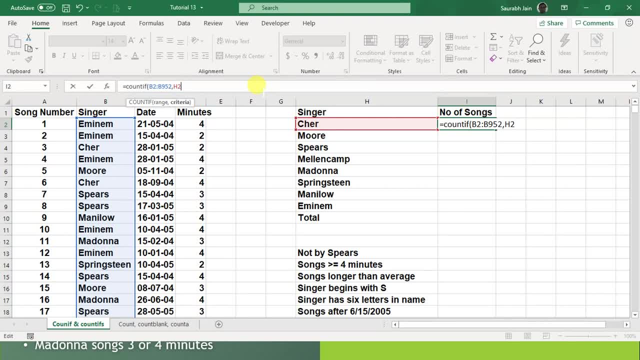 h2. fine, now bracket close and i press enter. so i came got 112. remember one thing: it's a one special thing: p i have to apply this for same also. so if i do drag like this- though we have discussed the relative and absolute reference thing- my data cell has gone down, if you see, my range has gone down. so 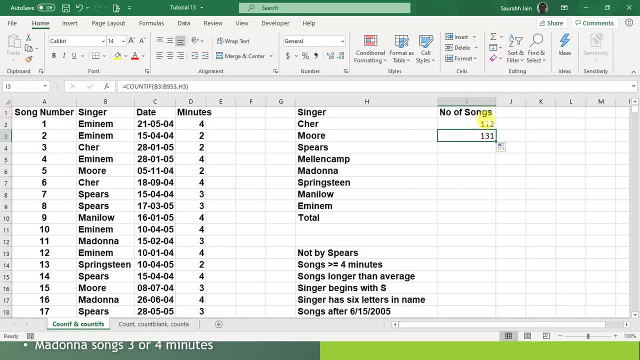 i have to freeze my log through this range, so what i need to do is in this, when that was my range option, I can just press F or so if you'll make it absolutely so now, this will be perfectly fine. now, when i apply, it will give me the right ready. 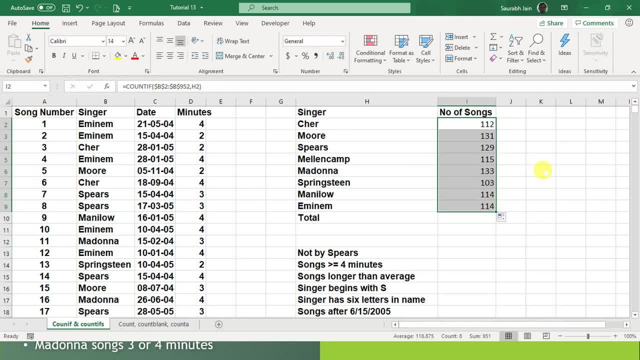 Did I say I' ll check, Let's see. So now I applied, when I use this formula at the same range available, because range is every time same. you will press the dollar signs and make it an absolute referencing, and then we will use there's. 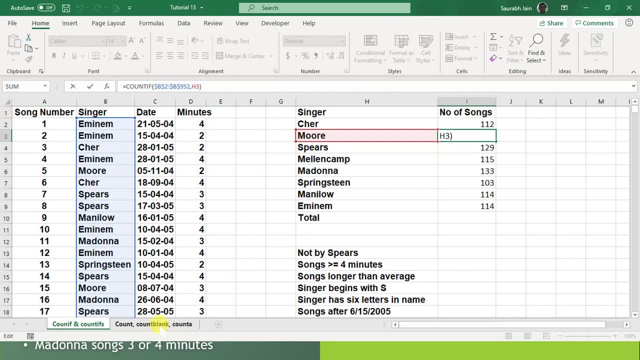 another way that we can name this range with our name functions. I'll take that in a separate chapter tutorial, but this is the way it's been done, so you all know how to do total. we can press alt equal to, also alt equal to enter. so they have 951 songs in which madonna has sung 133. fine, so 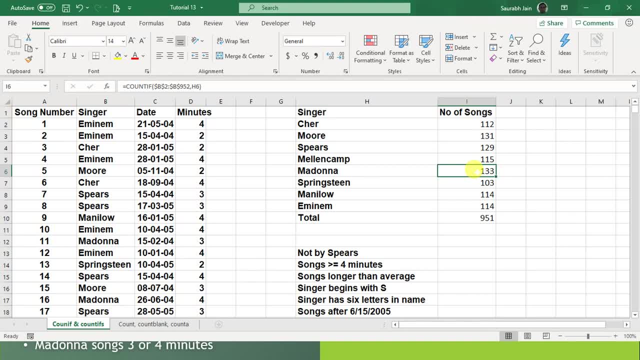 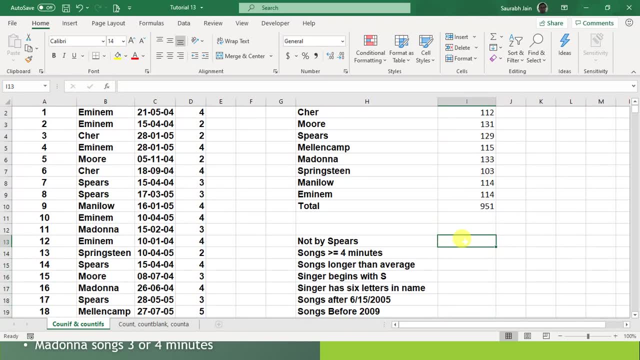 this is how we use counting formula. so this was the first question. now let's take another questions and try to answer these. I need all the songs, but not by spares. fine, so what should be the actual answer? I have total 951 minus 129, right? this should be the answer. so if I just try it out, 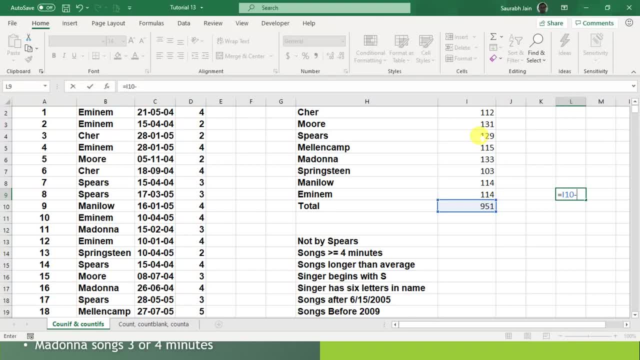 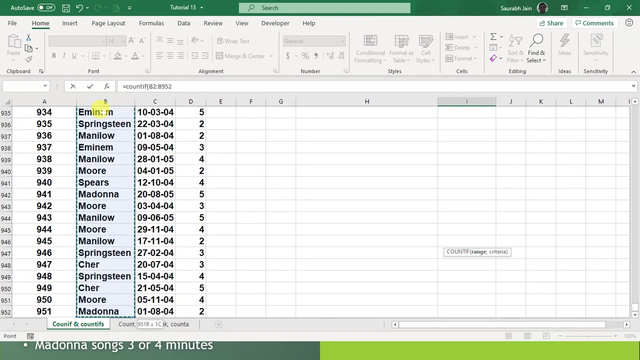 is equal to 951 minus. this is the answer I'm looking in this cell. so now I have to apply a count if formula again to solve this question. so let's see: is equals to c o u n t. count if bracket open. this time I say count if again the same name ranges, but this time I don't want to take. 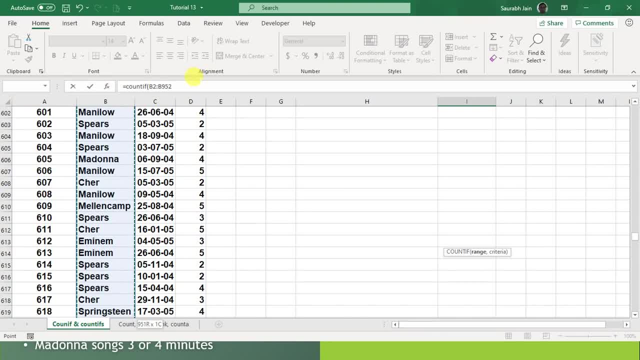 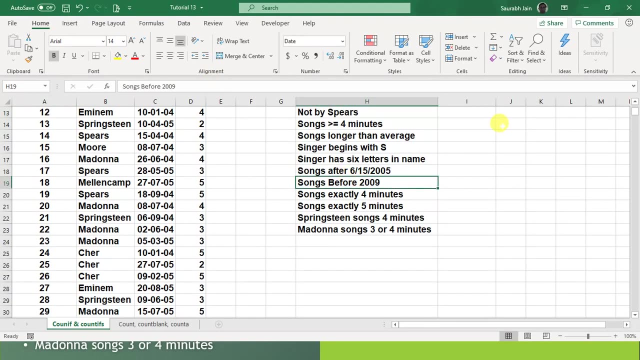 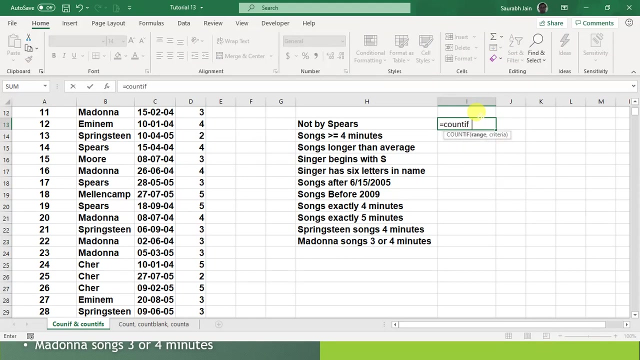 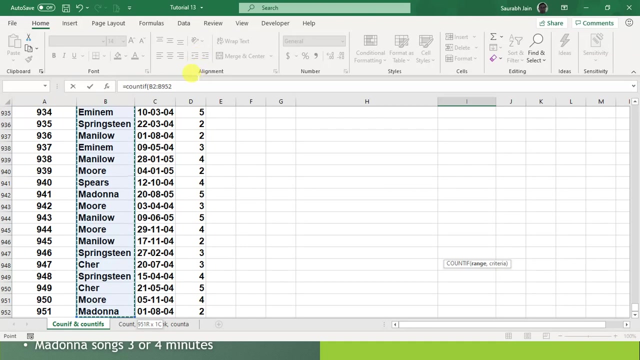 spares with me, fine. so my criteria is: I'll say comma and I put inverted commas because I want to put a condition. sorry, let me do it again. s? p e r s is equals to c? o u n t count. if bracket open, I selected an arrange, I put comma. 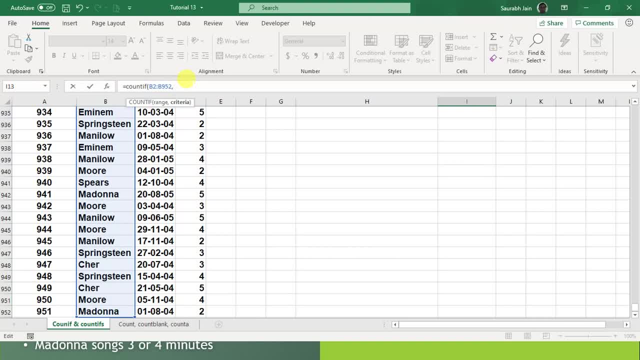 now, in the end I'm going to put a comma and I put inverted commas because I want to put a condition: the inverted commas, I will say not equal to inverted commas. this is the first less than sign and then the greater than sign. so this is called not equal to and I'll write spares. 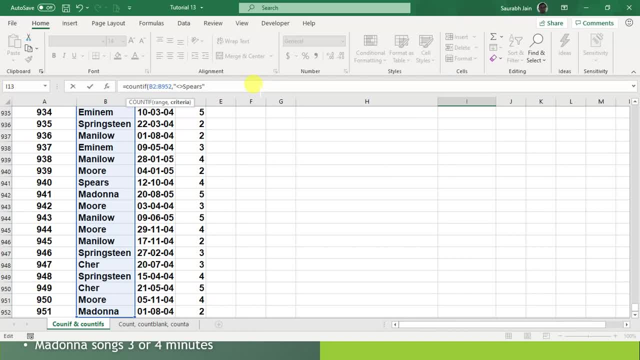 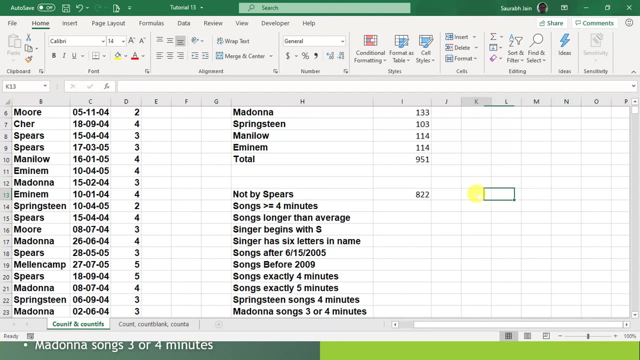 now I'll close the inverted commas because, uh, spares is not equal to both our x content, so we have put in the inverted commas. now I close the bracket, enter, so let's see what the answer. so I got the answer 822. yes, this was only i was looking forward. fine, so this is the first answer. now i 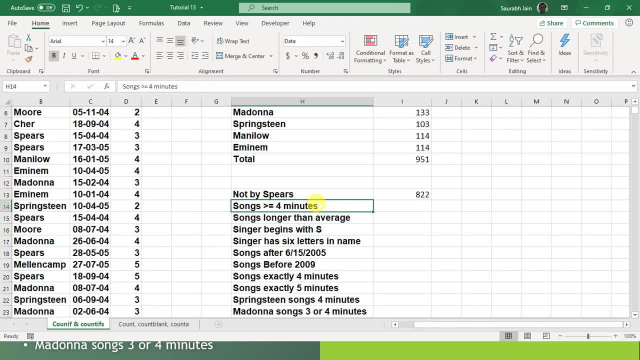 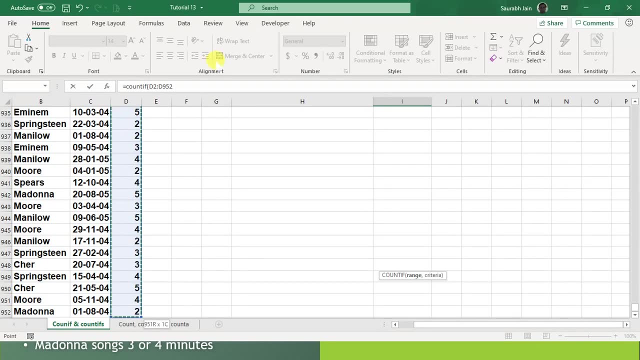 have a second question: which are the songs greater than equal to 4 minutes? so again, i'll apply the same formula: is equals to count if. but now i will select from our minutes range. so this is my range, i have to count from this range. i say comma and this time inverted commas. i say greater than equal. 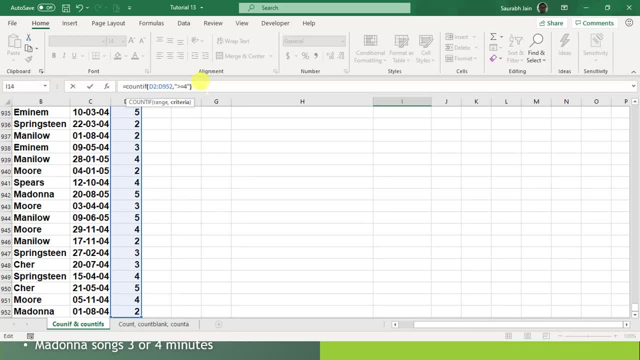 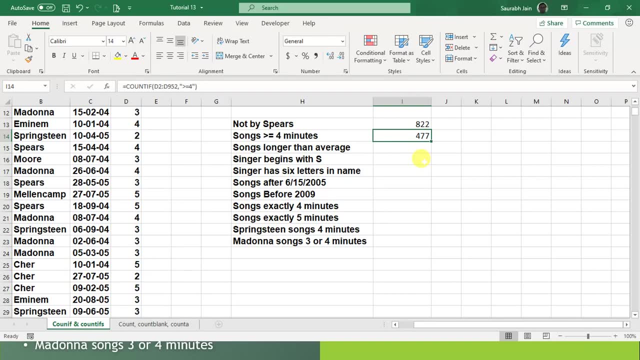 to four. fine, and i say: like it, like this, let's see. so i got 477 such songs which are greater than equal to four minutes. third songs longer than average. so this is the same formula. actually, what i need is i need to calculate the average also. 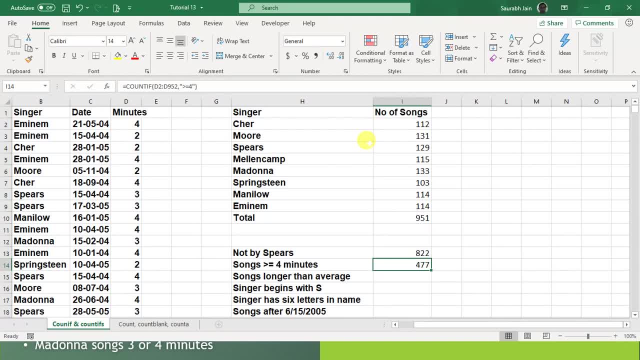 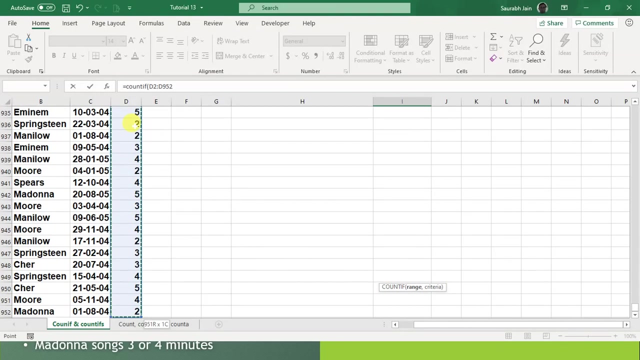 now there are two ways. i can just calculate the average in some way and compare it like this, or i can just choose the formula let's see how i'll use. is equals to count. if bracket open, i have two songs longer than average. right, this is like first, my range. 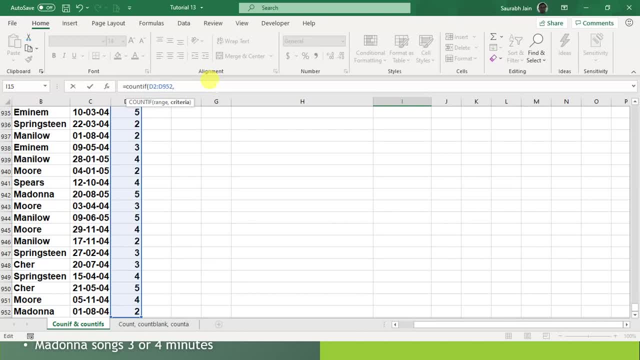 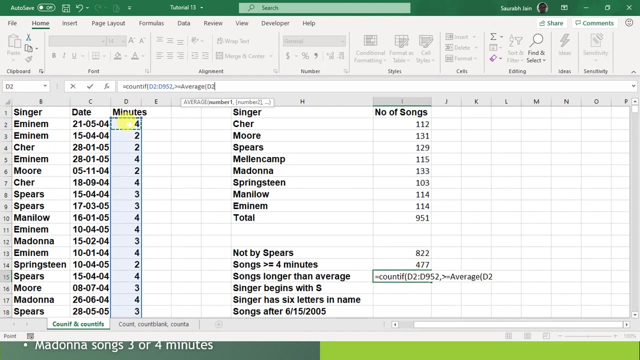 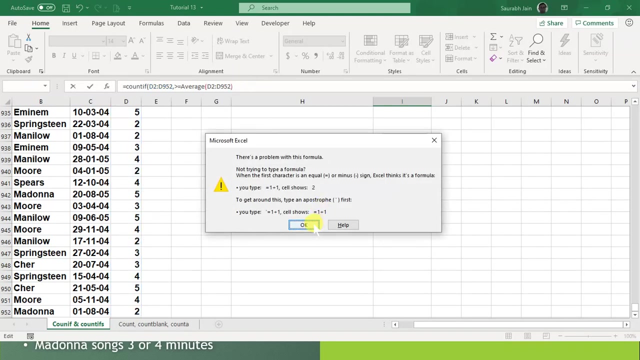 comma. now i have to take greater than equal to, so i push greater than equal to and i say average, so it has to be like a v e r a g average bracket open. now again i use and i do the bracket close. so now this one thing: you say greater than equal to, so you put inverted commas. 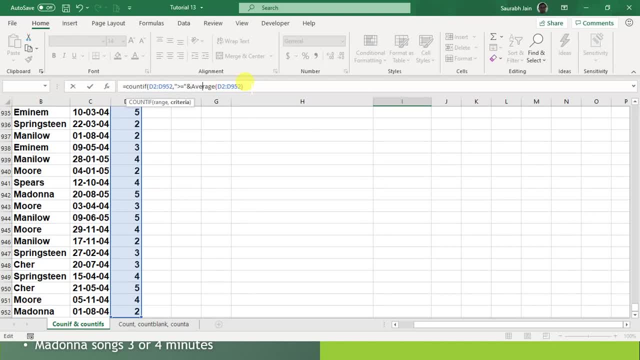 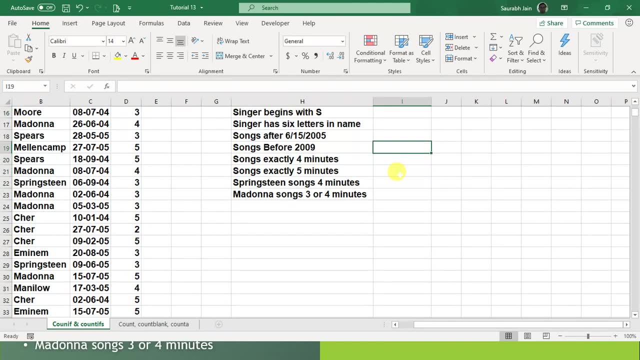 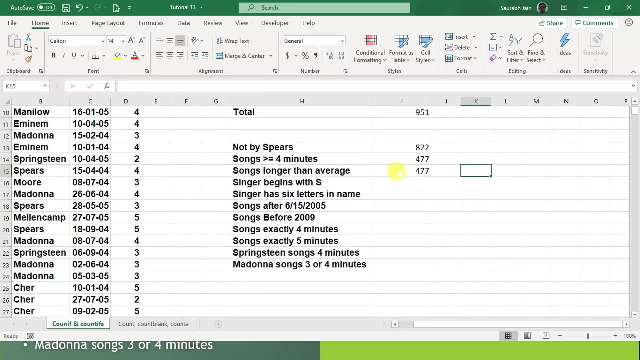 and to join it you can use ampersand sign to make it a formula. so now you can close it out. so you got answer. let me explain again. so songs longer than average is also same. to see this formula it's getting. See this formula is equals to formula text that we always do. let me take this formula. 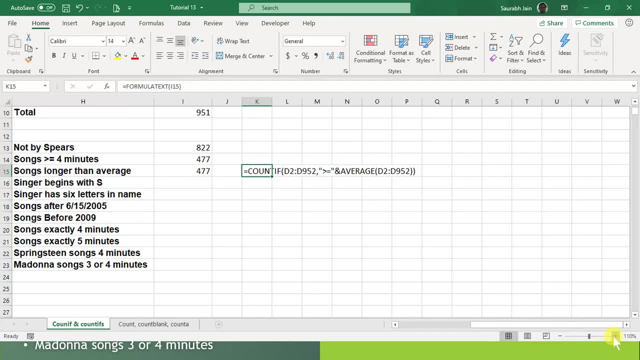 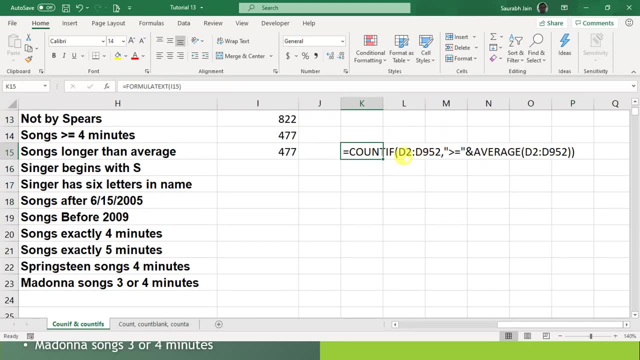 What I have done is see this formula. I will just zoom it out for you Now. if d2, this is my first of all, what we say- range now greater than or equal to, has been in the inverted commas, and I have used ampersand sign to connect this value average. 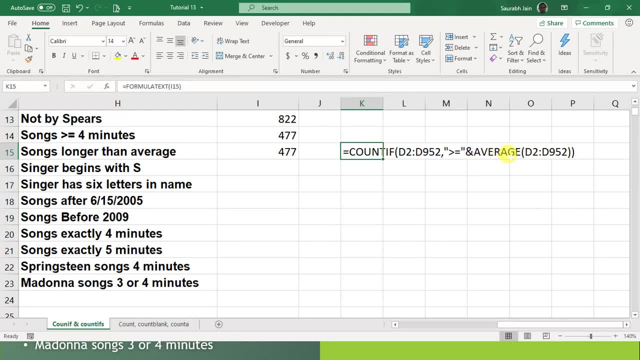 because I need to calculate the average also. So this has been lying like this. fine, So this is very easy. this ampersand is used for concatenation, you always know it, and it has to be outside the inverted commas so that it can join up, fine. 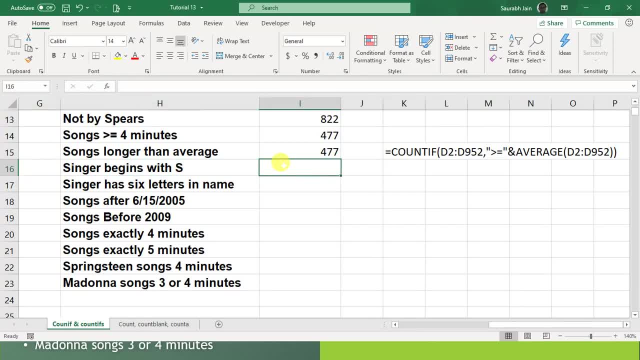 Now this: Okay, So this is another one we need to identify. we need to count all the songs with the singers whose name begins with S. So what you need to do is there are two wildcards. First is wildcard is called S trick, which implies that star means anything and there 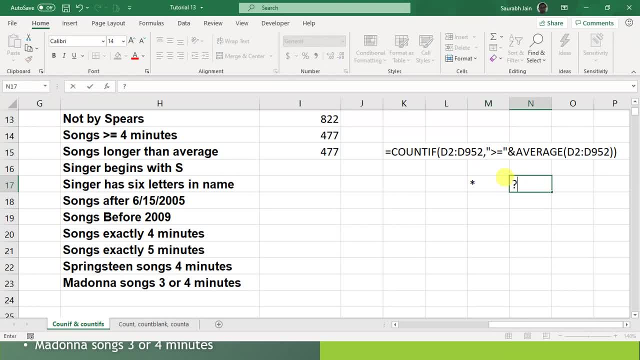 is an ampersand question mark which says anything in that position, So I will try to explain you how it works. let's first solve this one. I need to identify all the singers. sings with S. So is equals to countif bracket open. 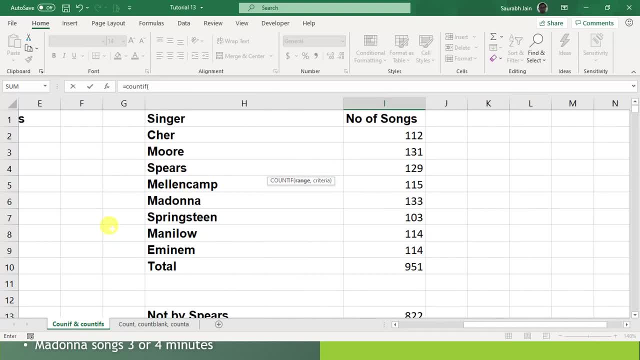 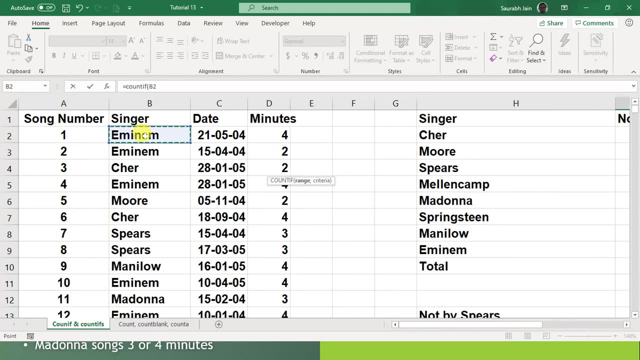 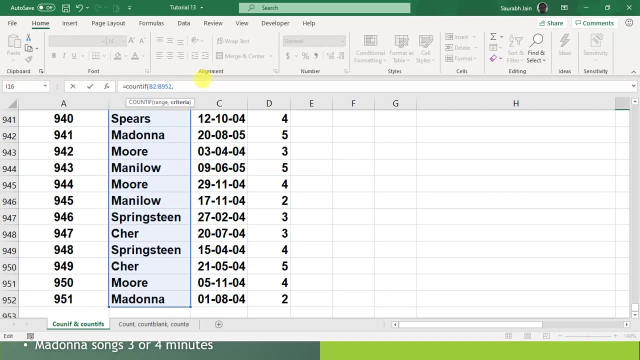 So now, where are my singles? So this is my range. So now criteria has to be what Criteria needs that? it should be Okay. So Okay, I want to identify all the singers. So here is the criteria: I want to identify all the singers. 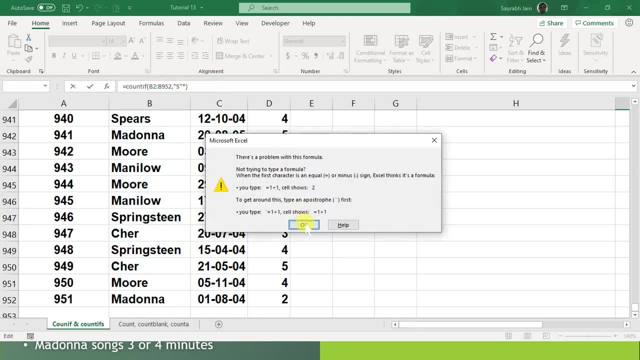 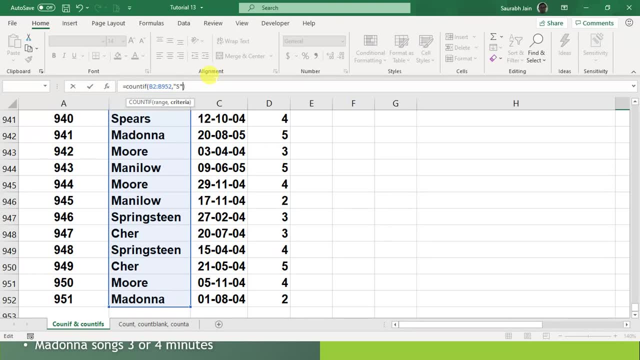 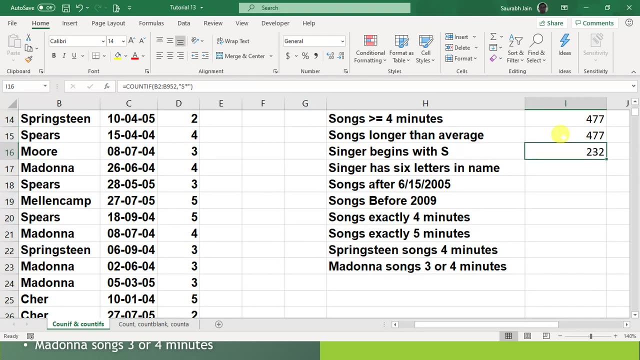 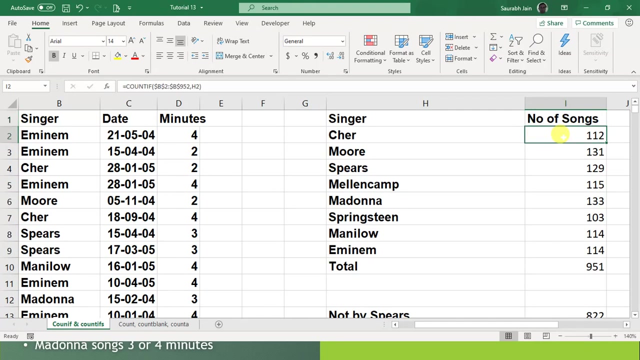 So I have put it there and I've put, I've put S and I put ampersand sign. Let's see, Okay, I forget to put this, The star, and then it won't. So here comes Singers, whose name were with S. Let's see, Spears was with S. There were two names, Fine, 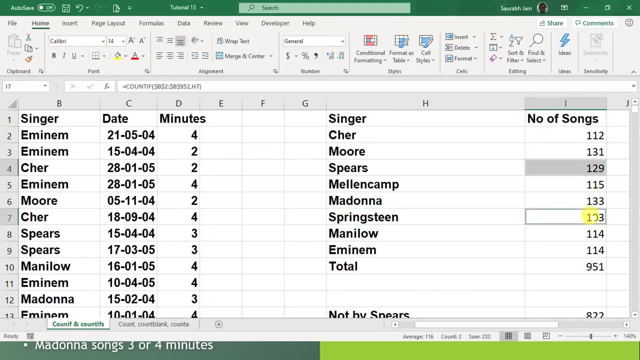 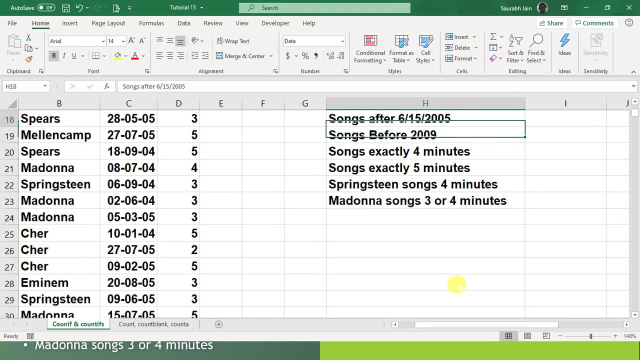 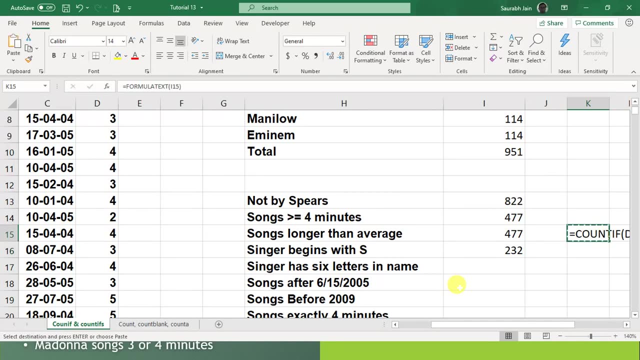 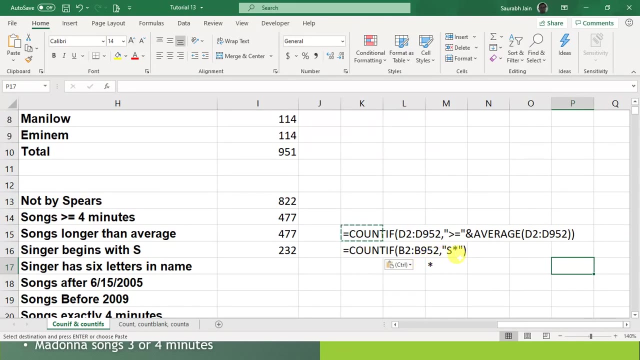 129 and 103.. So that comes to be 232.. Fine, So we have got the correct answer. What I have done is I will explain you again. See Count if comma S and star. So first letter is S, which is mandatory. 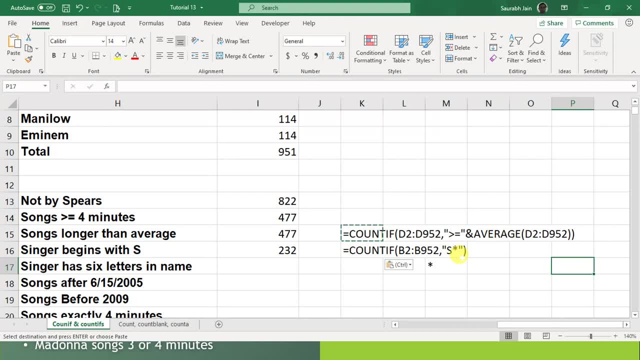 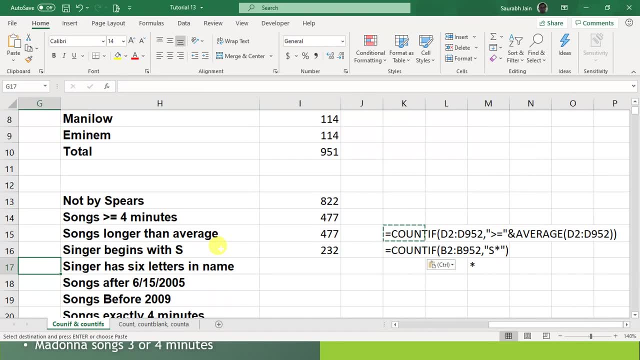 and after that it can have any number of characters. We have just put the asterisk sign over there, So this is how we can. we were able to do. Singers begins with S. Now you have a singers which has six letters in name, So now we have decided that it has to be six letters. It can be anyone. 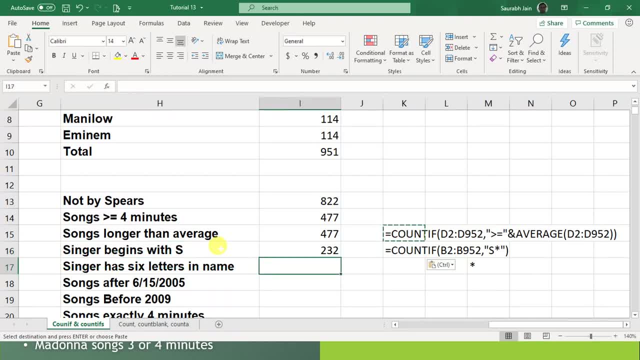 So instead of that, we will use a question mark, I will just control C. What I do is I will just put control C. Let's go over here. So now, this time, instead of S star, we will use six question marks. Our question is: count all the names of a songs? 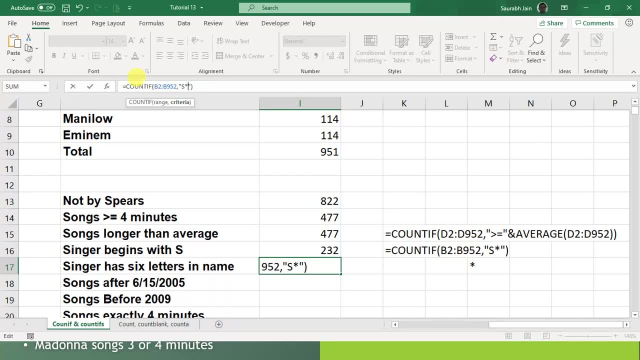 Whose singer has six letters in name, So a, 1,, 2,, 3,, 4,, 5,, 6.. So I have put six question marks and I press enter. So this is 243.. Fine, Control C, Control B. So I have put in inverted commas. 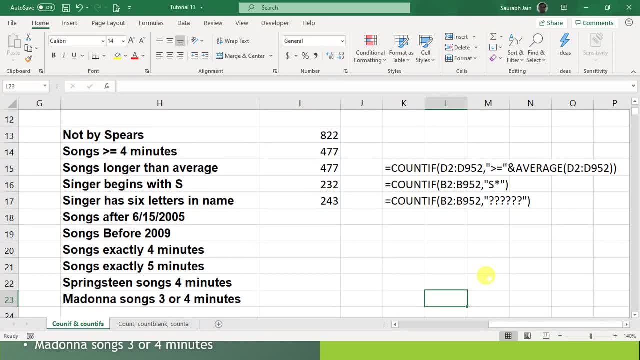 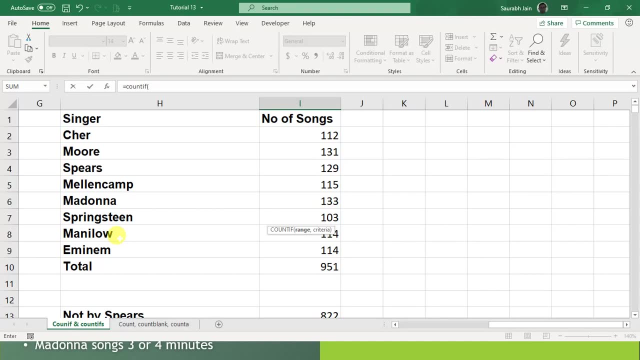 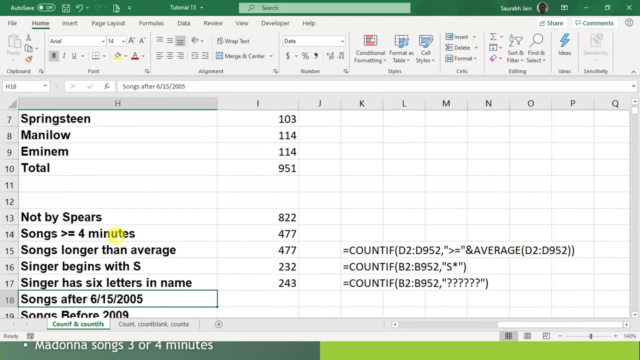 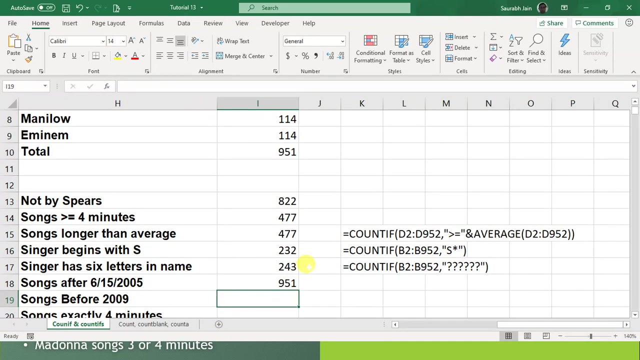 question marks. So this has been able to give me the result Now, which are songs greater than 650 in this? So again, what you have to do- You have a date available, So you say- is equals to count this bracket open Songs after this, So greater than 6 by 15 slash 5.. So here is my answer: That's 950. 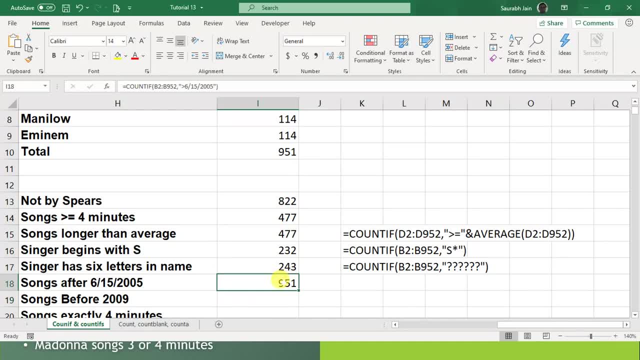 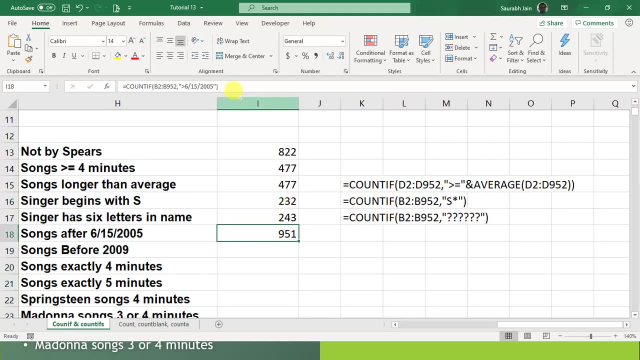 and all words after that, Fine Songs before 2009.. So you can again do the same thing. Control C. This time you can say 2009 and I have done it one, I have taken one date and instead of 950 and all words after that. So I have done it one, I have taken one date and 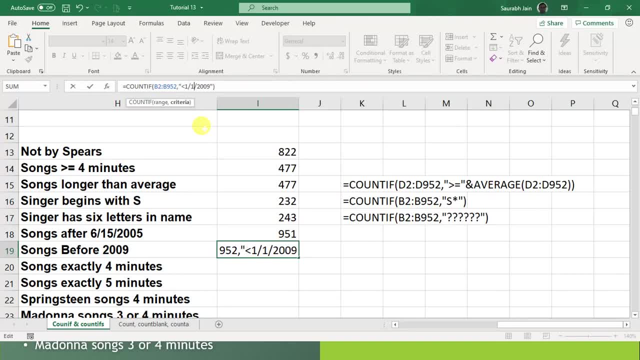 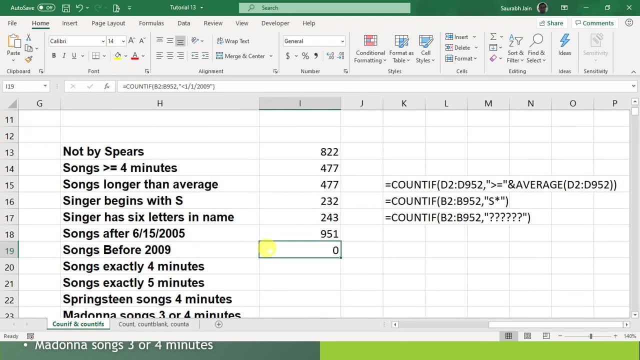 instead of greater than I have to choose less than. This will also give the same answer. What I've done: Songs before 2019, right. So I need to check what criteria I have taken. why did the mistake? my criteria was wrong. I have to take from date one, right. 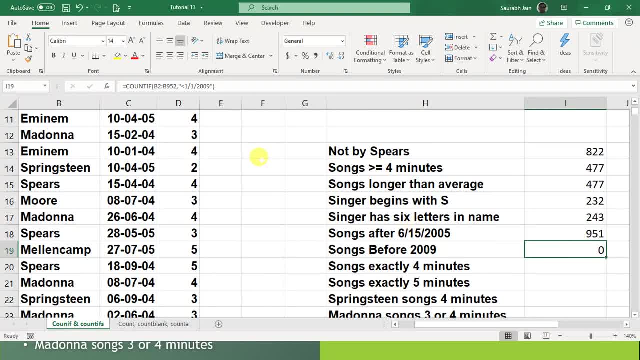 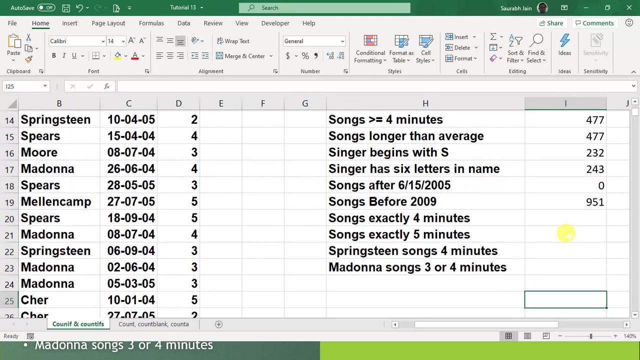 so that's why it was coming wrong. so I will do this by this. I will apply the formula: instead of P, it will be C, C to the answer right here. also, I will use the same thing: mistake C, C. now let's talk about songs. exactly four minutes, so now I need to identify the. 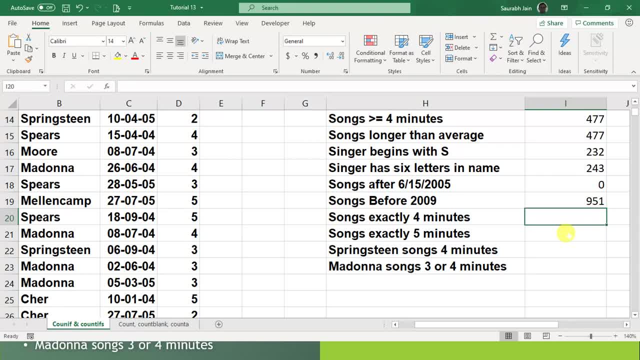 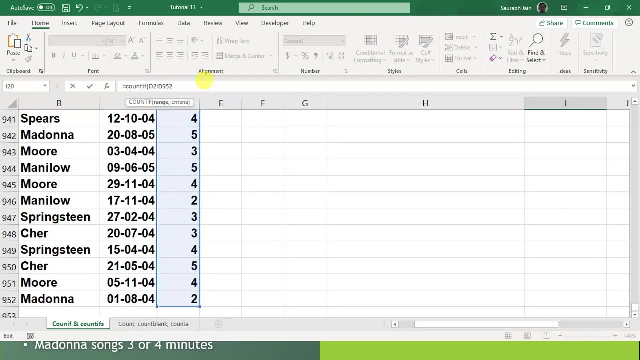 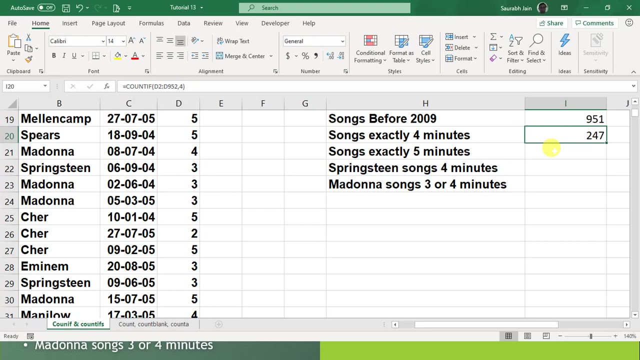 songs which are exactly four minutes. so this time it will be equal to four. fine, so what I do is equals to count. if bracket open, I again count the which are equal to four minute. you do this and in comma you put four and bracket close. so here comes 247 songs which are exactly four minutes. now let's do song exactly. 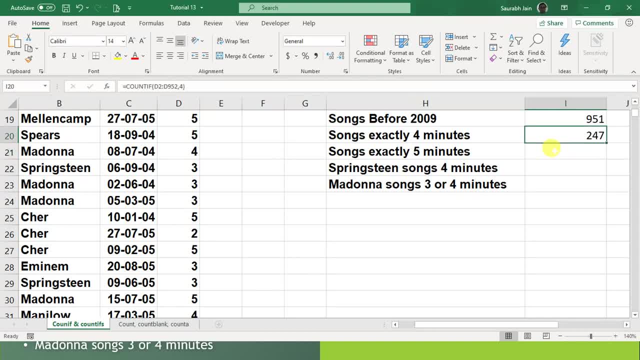 five minutes. it's the same thing. control C, sorry. so what I want to do is that, see, this time I'll put control B. this time I need exactly five minutes, fine, so I have two thirty songs now. there's another question now. till now we have done a. 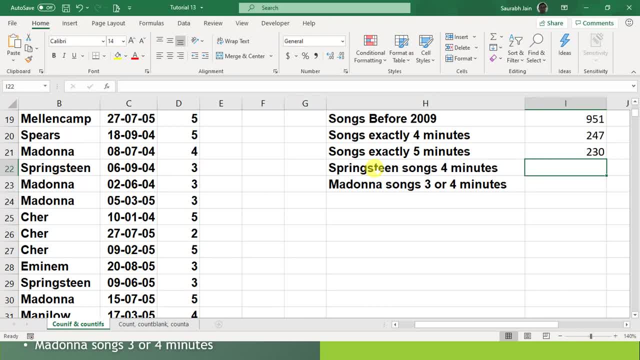 count. if now we want to go of count, if there's a multiple criteria, that what I need to do is explain. the string has songs which are of four minutes, so what I want to do is that is equals to count ifs. I'll use count ifs formula. I'll say: 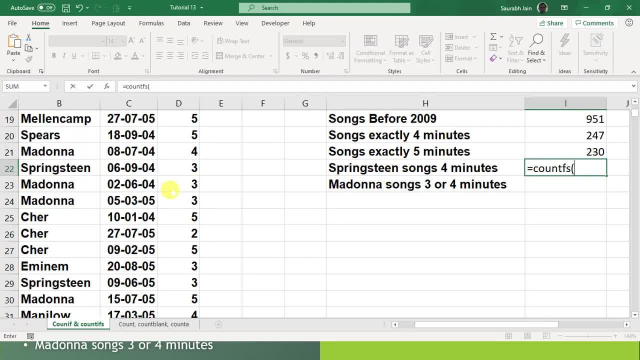 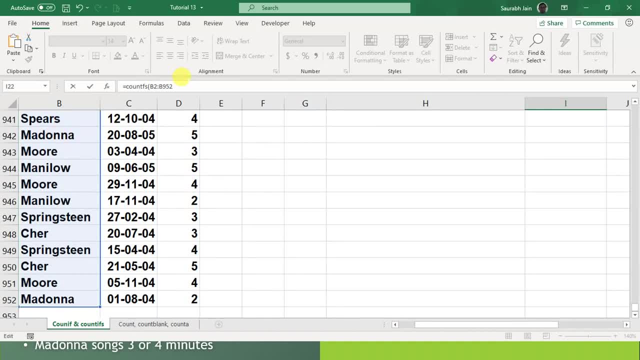 bracket open. fine, now first I have to need to explain string, so I'll say again: right area I put comma and in inverted commas I write S P R I N G S, T, double n springsteen. so this is my first range and criteria. now I have to do for second. 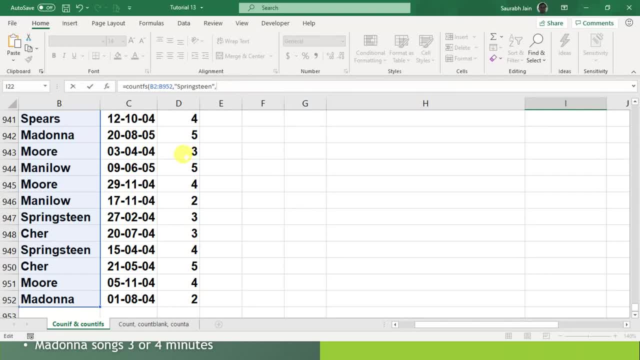 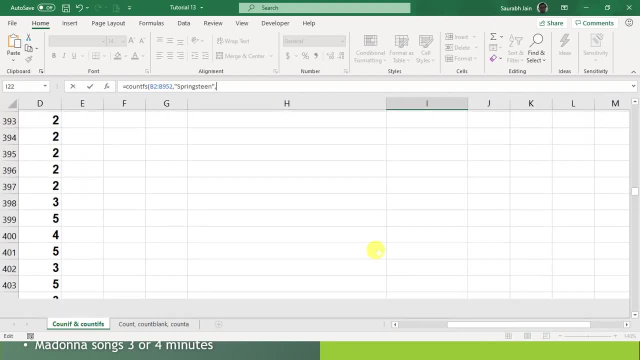 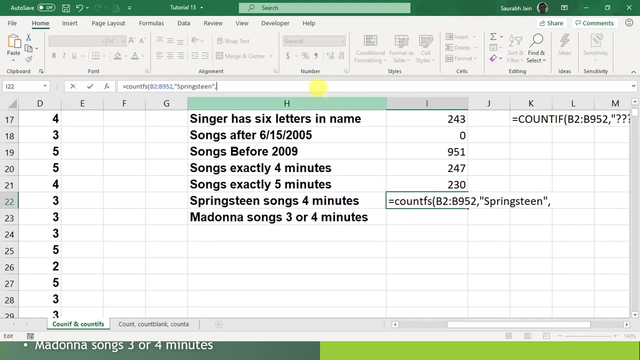 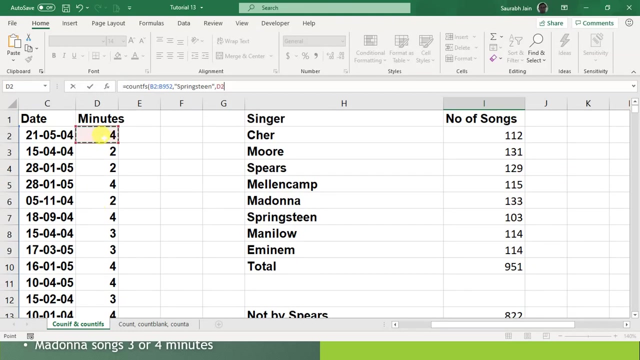 range, and second criteria for which I'll do is comma. now my second range is what? what was my question? songs equals to four minutes. so I'll do second range, which is like: this is my second range: comma. and now it has to be four minutes so I can write four and I 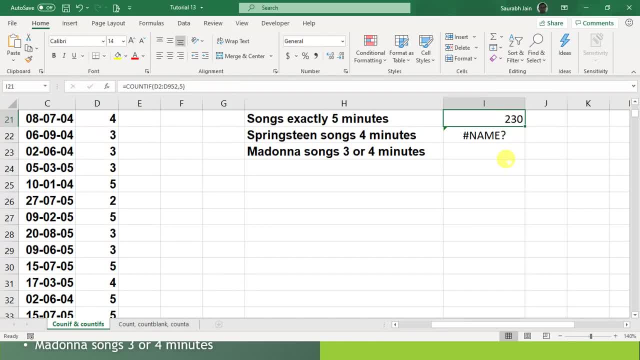 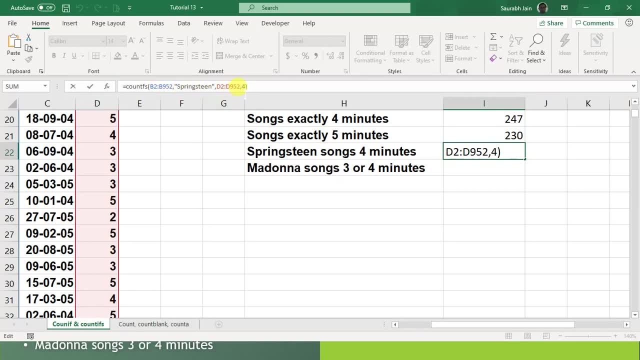 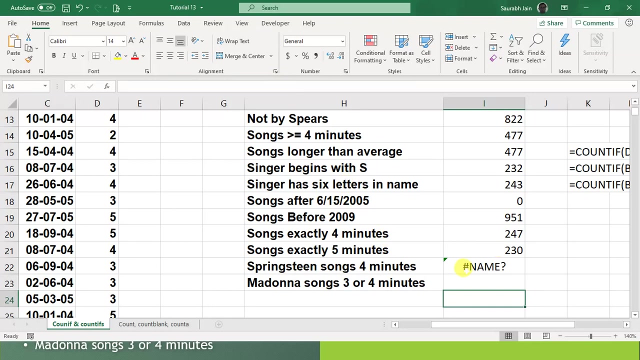 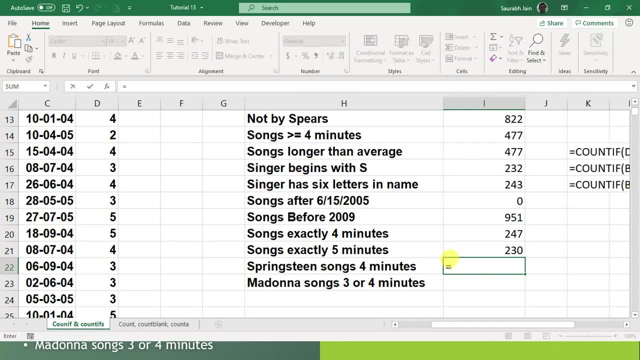 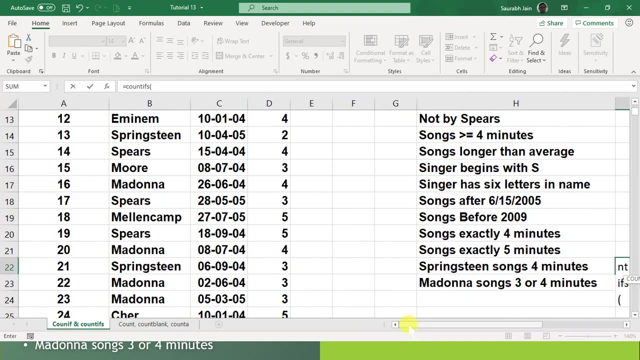 it's like B and then is it like B. it should be correct for what I went. why did see? let me c o u n t count ifs bracket open, so i have to criteria range one. so my criteria range is that this has to be the name, has to be from this cell. 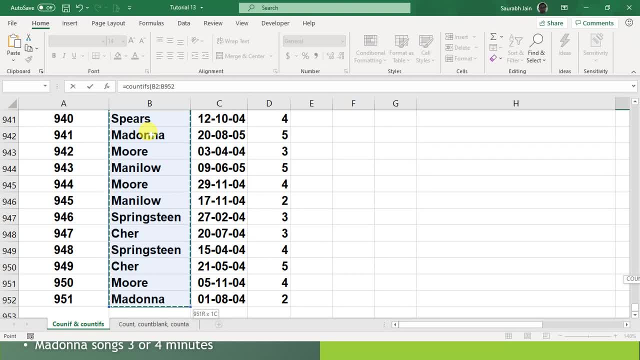 fine, okay, now i have to apply comma. now i have to apply inverted commas. and i have to apply s p? r i n g s t w n springsteen. now i close the bracket. inverted commas. now i have to apply range. two criteria: comma. now. this time my range is for four minutes, so i just move ahead. 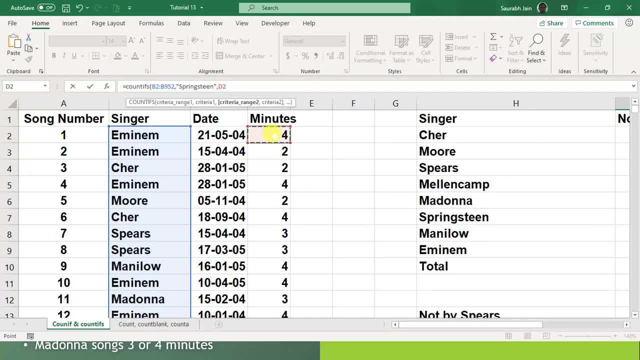 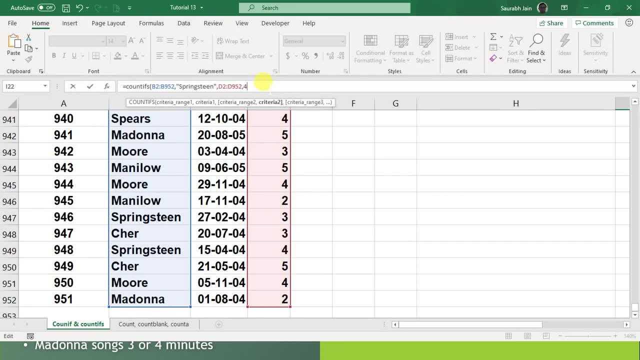 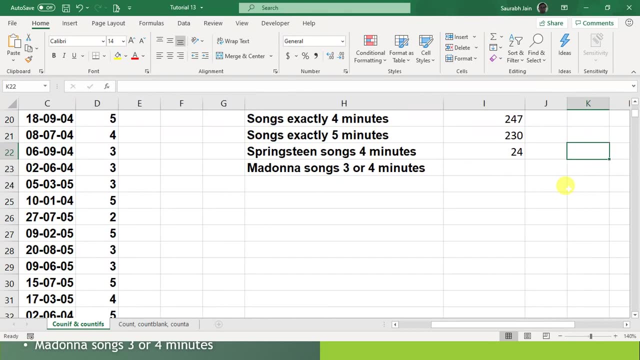 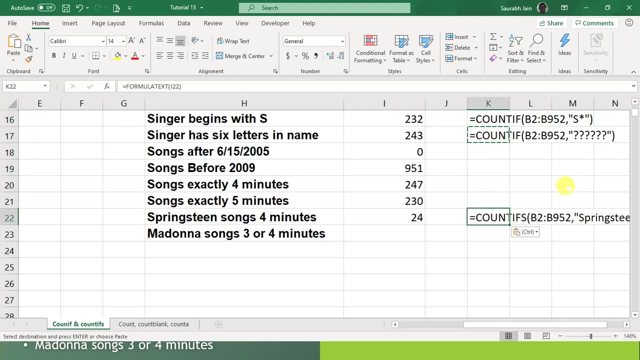 and i'll take this one. so this is my range. two: i put comma this time. say four. here comes answer. so it is 24 minutes. so if you need to understand this formula again, i'll just apply the formula for you: ctrl c. so c is equals to count ifs. 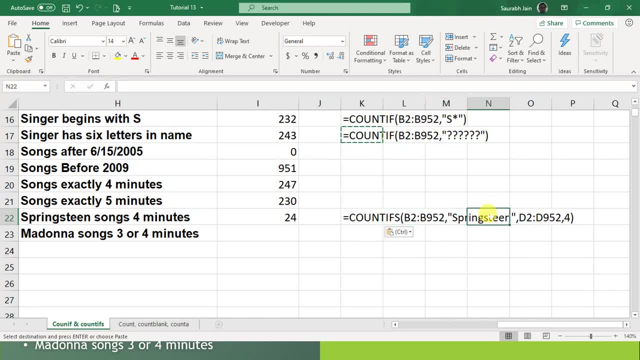 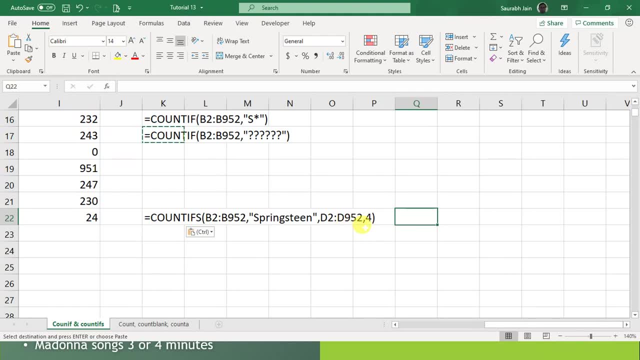 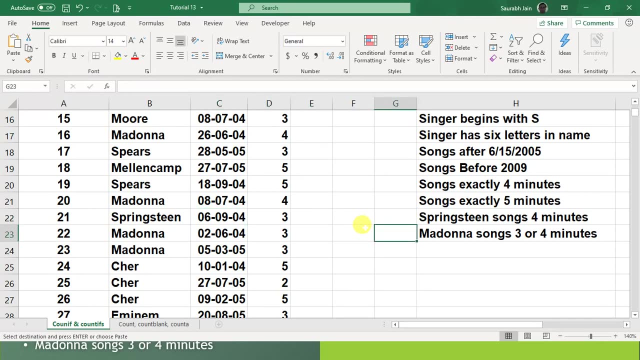 this first range, then your name and after that d2, second range. write it so like: Range 1, criteria 1.. Range 2, criteria 2.. Range 3, criteria 3.. Like this we can do these questions. Now you have another one Madonna song, 3 or 4 minutes. 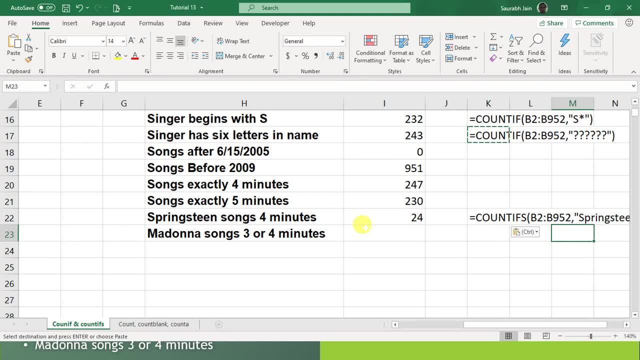 So now, this time you have to use the range three times. So what you need to do is first count ifs. In the name range you select the name and say it should be equal to Madonna, Then in second criteria you say it should be greater than equal to 3, and in fourth, 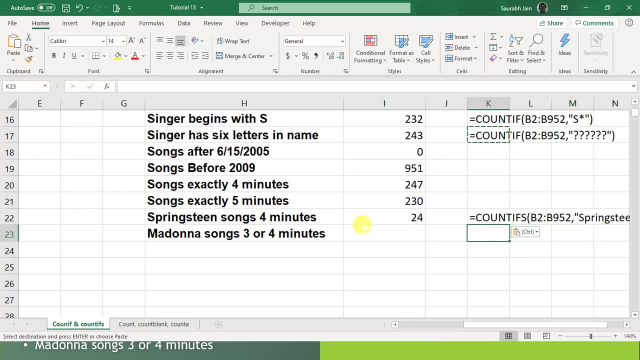 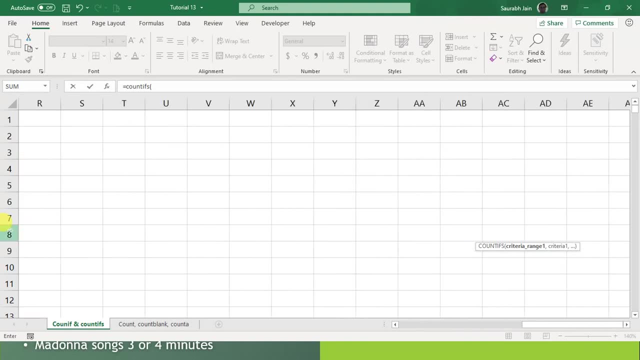 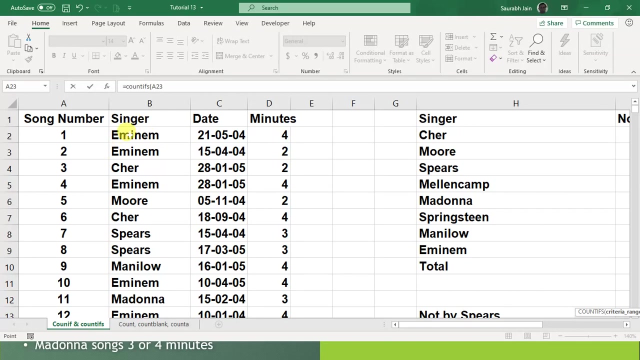 you say it should less than equal to 4, like this, So let's do it again- Is equals to Count. ifs bracket open, You have your range, This is your range, This is your range. Fine, And M A D O N N? A. So I say comma. 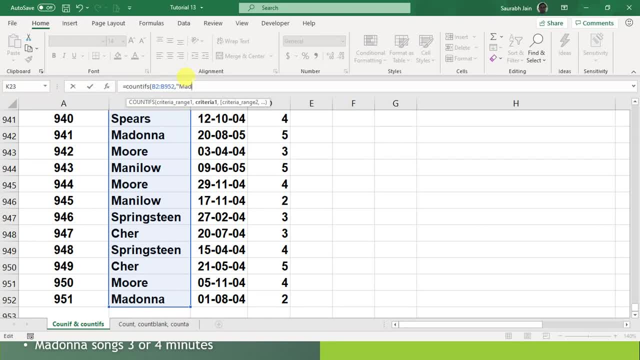 Invalid comma open: M A D O N N A Madonna. fine, So you will close the invalid commas. This is the range one comma. Now you have to do the criteria number two. So this is your range Now. this time you will say: 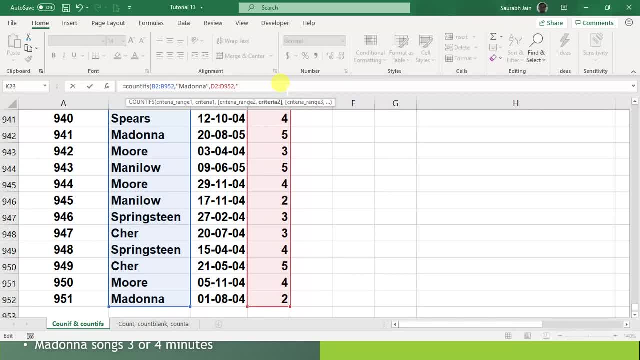 Comma, Invalid comma: It has to be greater than equal to 3. Close Comma: Now again you have to write a Range. This time you say again like this: and you should say again comma, and In invalid commas you say it should be less than equal to: 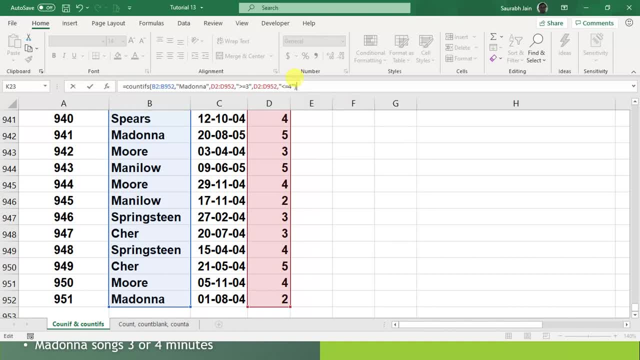 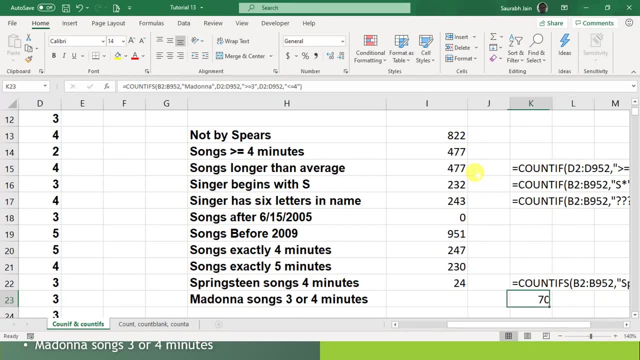 4. Invalid commas: close Black it and press enter. So this is your answer. Let's see I have used a different way. 70, fine, no issues. So you got 70 the answer for this. you can just put it again in copy-paste: 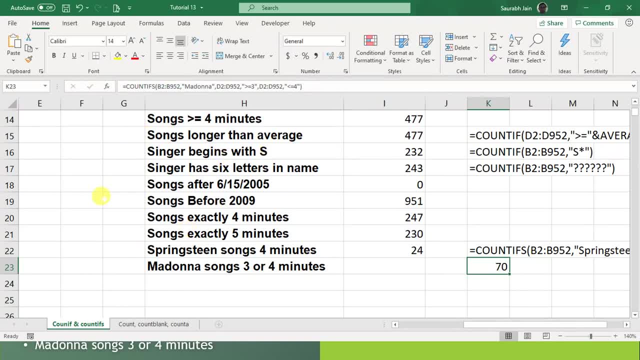 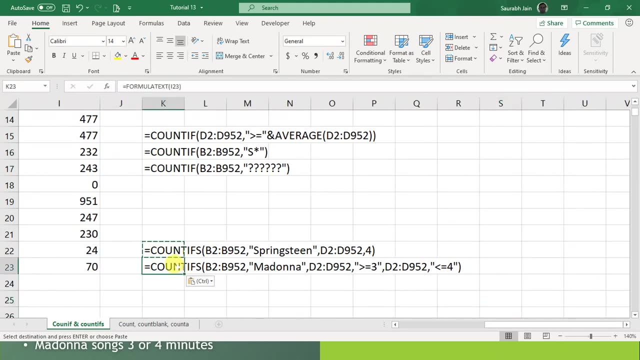 C copy And just put this over here, So you have 70 answer. if you want to see control C and control B, so see what I have done. so now this is counted: first range, then the condition criteria, one second range condition and third criteria. because it has asked. 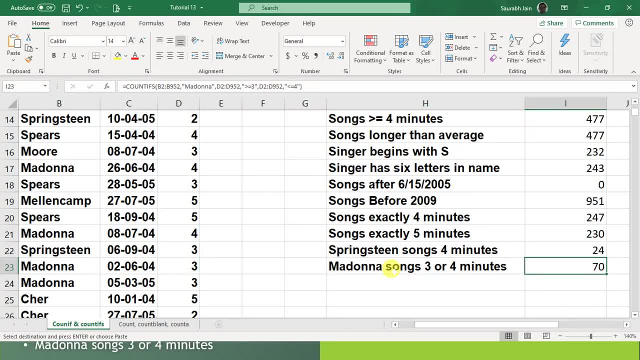 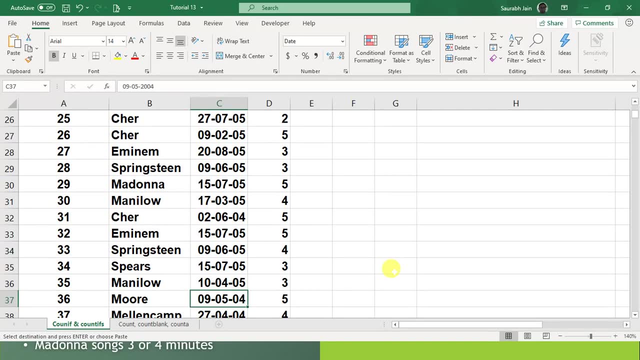 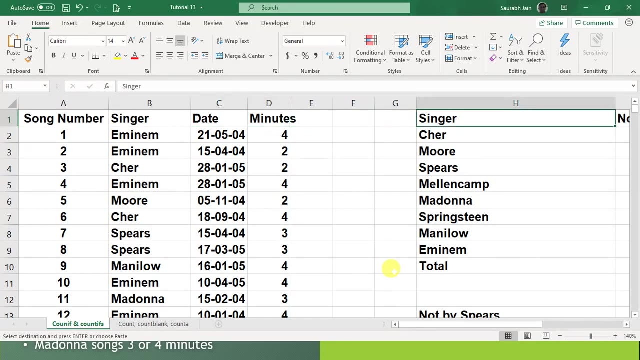 three or four minutes, so it should be greater than equal to 3 and less than equal to 4, so it will include 3 and 4 as well. fine, so this is like this. it can be done. fine, so this is the way we can use counted formula. so what you need to do is you need 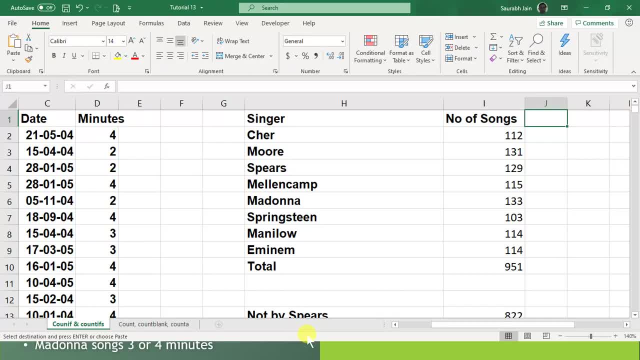 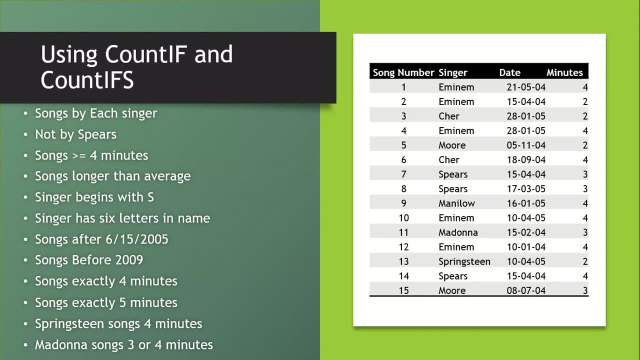 to download this file and practice it yourself. this is the way you will learn excel, because without practicing, nothing will happen. and I have a special request, if you are liking this course or if you are a newcomer- if you are a newcomer to this course, make sure you do the 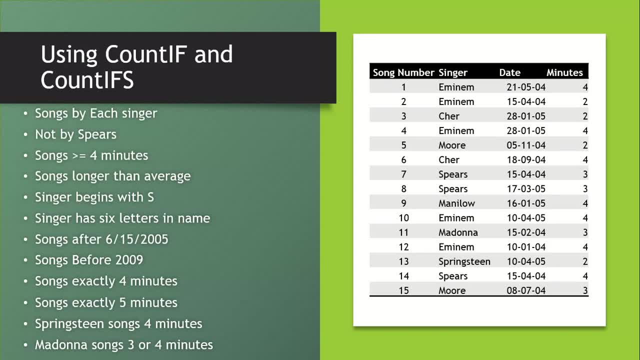 previous exercises. it is important to move sequentially with me and I am walking very slow. you can do it in, say, 2 to 3 weeks entire course. till now we have done so. this is important thing. second is: if you know someone who wants to learn excel, please feel free to share with.